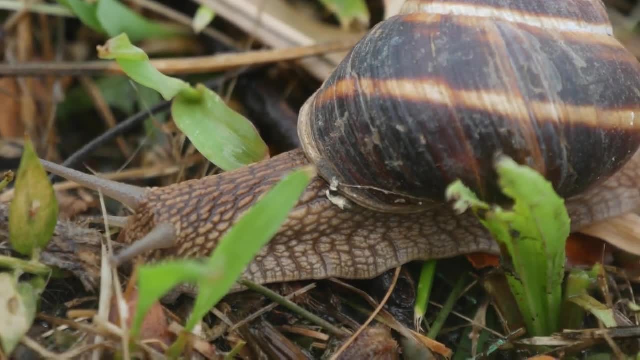 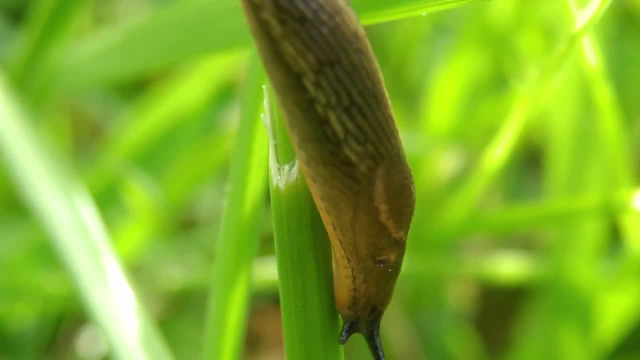 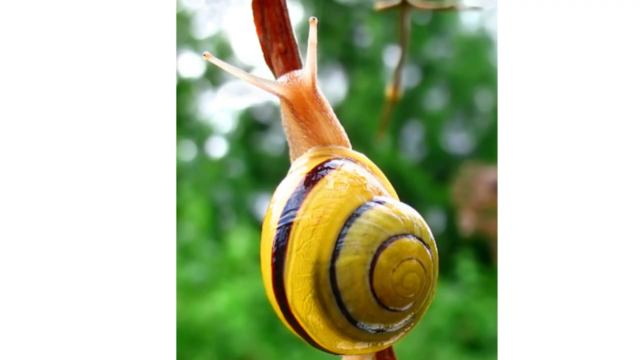 to members of this class. it is commonly used for those gastropods with an external shell. Gastropods without a shell are more commonly referred to as slugs. The class gastropods have a huge diversification of habitats. You can find them in gardens, woodlands, deserts. 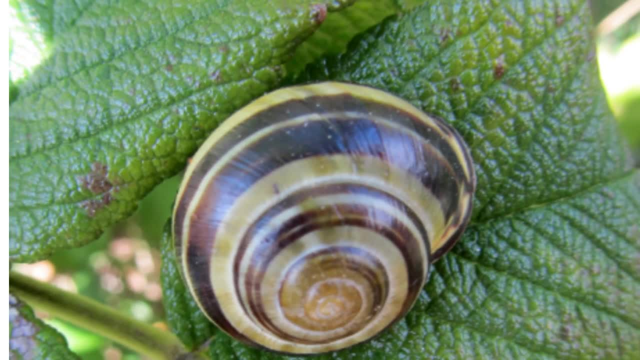 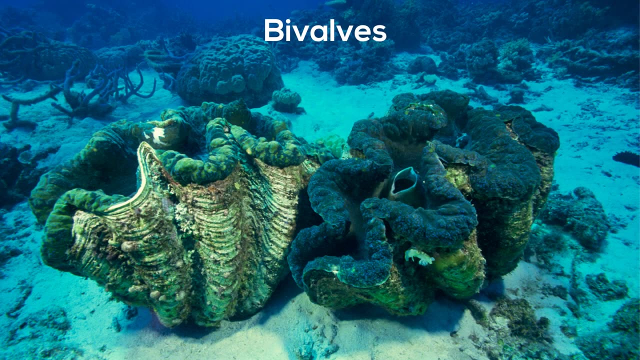 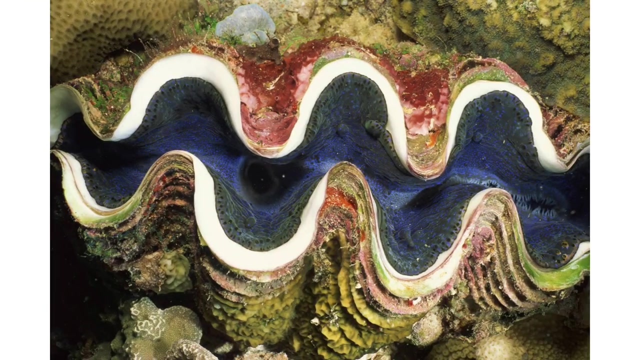 and even in the depths of the ocean. Examples include snails and slugs. Another class of molluscs are bivalves. Bivalves have two shells. Some examples include clams, oysters, mussels and scallops. They do not have a head and most are filter feeders. 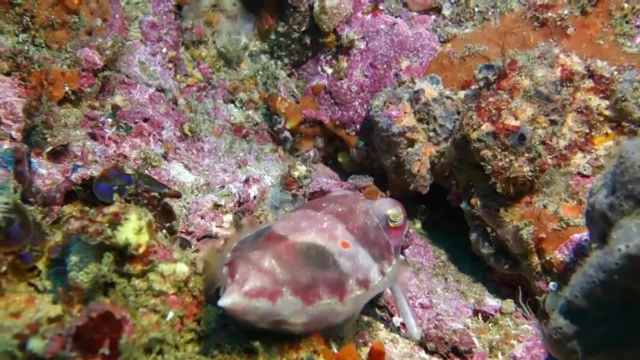 And finally you have the cephalopods. The cephalopods have a head and most are filter feeders. Finally, you have the cephalopods. The cephalopods have a prominent head, body & foot and usually a set of arms or tentacles. 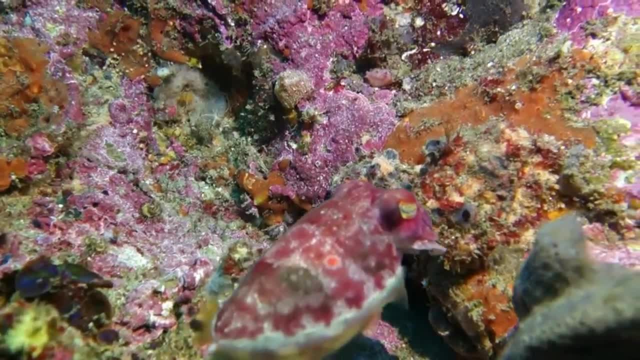 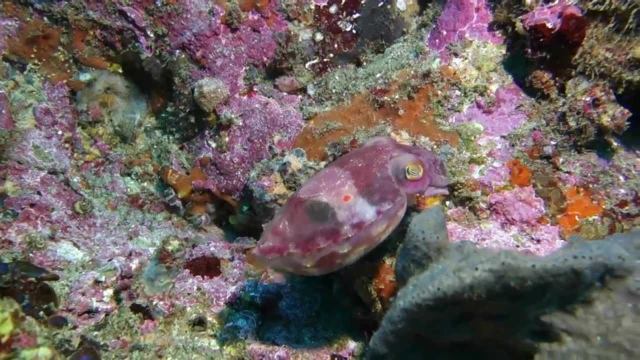 And finally you have the cephalopods. The cephalopods have a prominent head, body & foot and usually a set of arms or tentacles. Animals in this class are carnivorous predators and many of them have beak-like jaws. 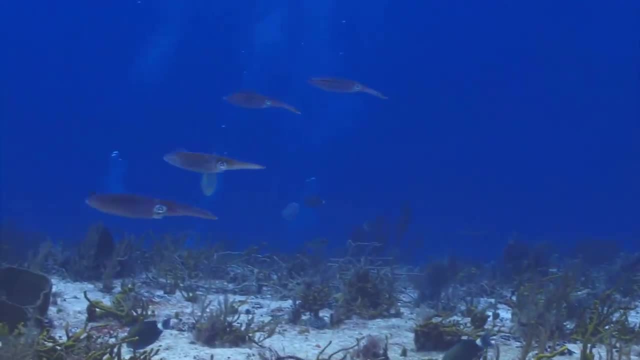 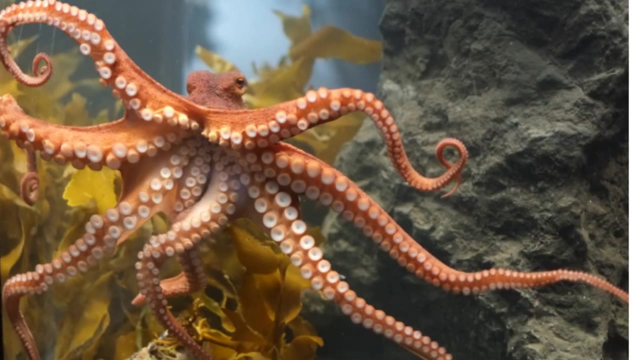 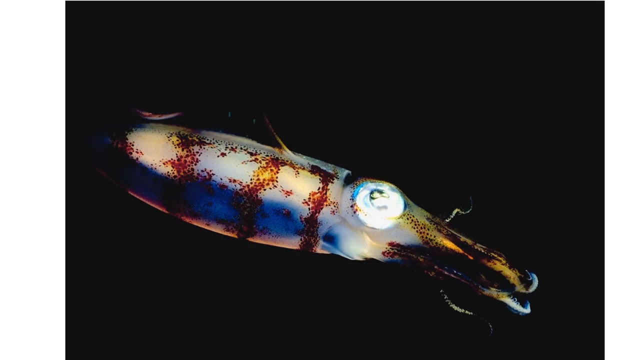 All cephalopods show a very well developed nervous system, along with eyes. Several can change colors very quickly or have very bright colors. Examples include octopus, squid and cuttlefish. The cuttlefish is very famous for having the ability to change its color. 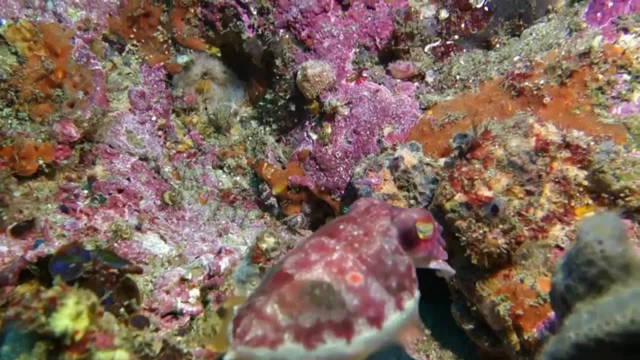 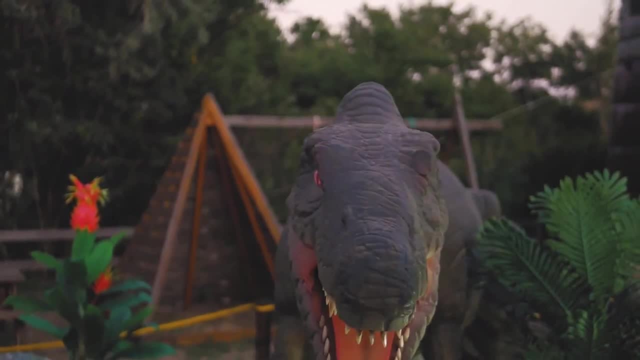 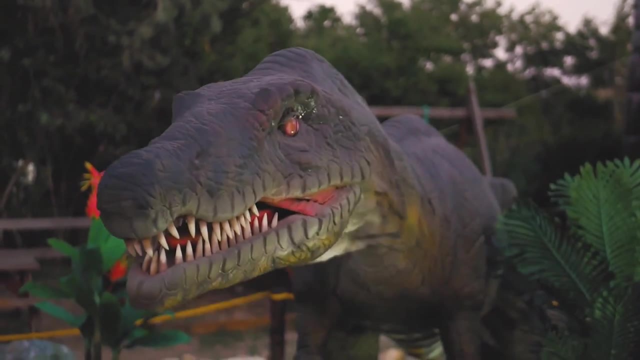 very quickly and to blend in almost any background. In the movie Jurassic World, the geneticists used the DNA of a cuttlefish in the abdominus rex and this allowed this genetically engineered dinosaur to instantly blend into its environment. Remember this was made up, Hollywood stuff, but it. 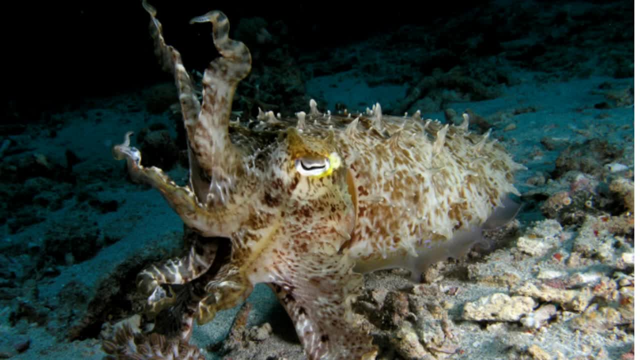 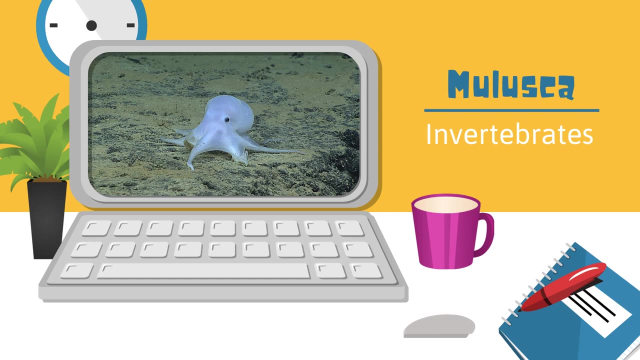 still was interesting. Although the cuttlefish appears to have superhero, almost Hollywood type abilities, it really can change its color very, very quickly. So there we go, a look at the phylum mollusca. Thanks for watching, and MooMooMath uploads a new math and science video every day. Please subscribe and share.